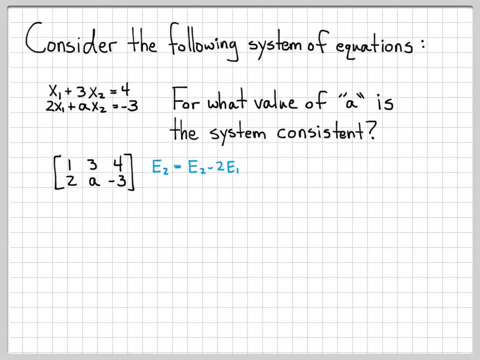 equations and do the same type of operations that we're used to doing, though We can still manipulate this into a form that we can try to solve the equations for. So let's go ahead and do that. Let's go ahead and let this second equation equal itself minus 2 times the first. So I'm 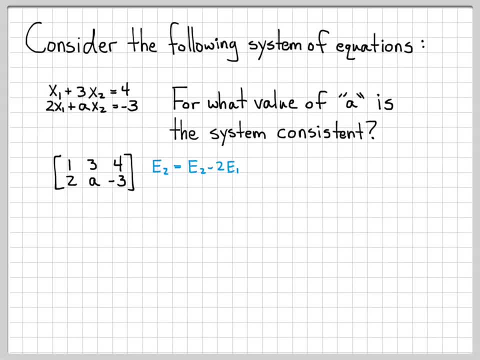 going to try to get a 0 right here, just like I always do when working with systems of equations in this augmented matrix. If I do that, then I end up with a 0 there, Then I have a minus 6 here, And then I'll have a negative 11 right here. So if I look at this equation now, if 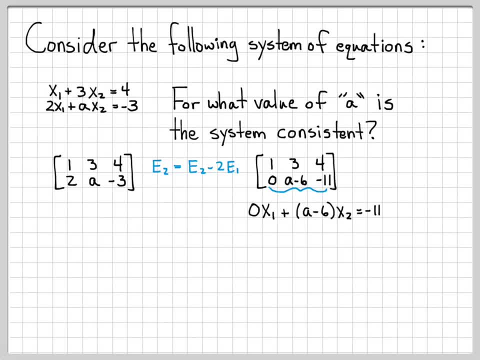 we write out what this means. what do I have? This equation says that 0x1 plus the quantity a minus 6 times x2 is equal to 0x2.. A negative 11.. Well, 0 times x1 is just 0. So this just simplifies to the quantity a. 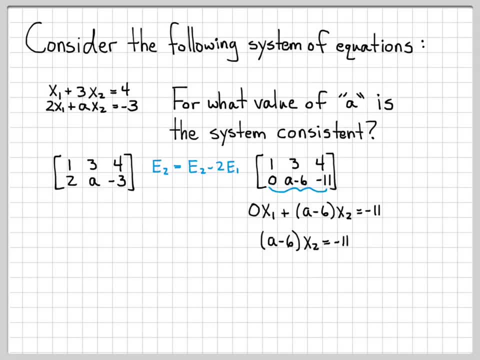 minus 6 times x2 is equal to a negative 11.. So the way I like to think about this is what would happen if this factor, a minus 6, was equal to 0? So if this term right here was 0 in its totality, I'd have 0 times x2 equals. 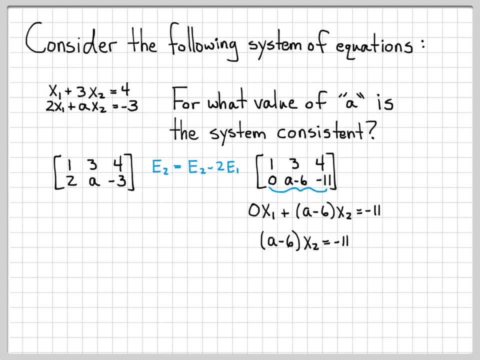 a negative 11, or 0 equals a negative 11.. So I'd end up with a contradiction. So I can't have a minus 6. equals 0.. Another way to think of it is if I was to solve for x2 by dividing this side of the. 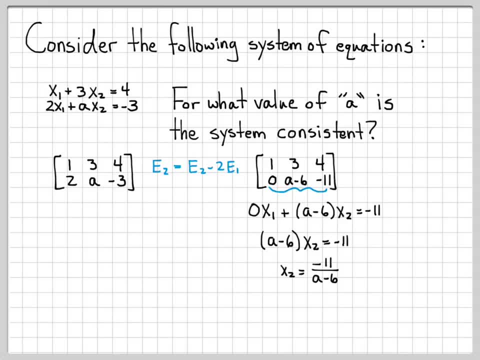 equation by a minus 6 and dividing the other side of the equation by a minus 6, I'd end up with this expression right here for x2.. x2 is equal to a negative 11 divided by the quantity: a minus 6.. 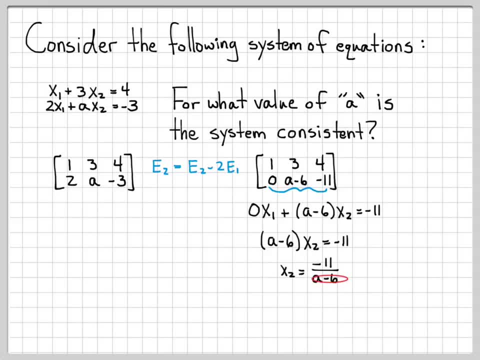 Well, obviously I can only do that division as long as a minus 6 is not 0. So same condition pops up. I don't want a minus 6 to be equal to 0. In the first case I would have an inconsistent. 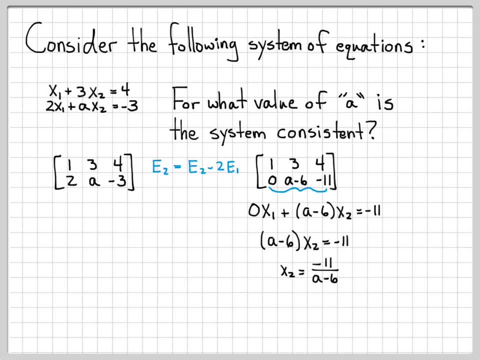 equation: 0 equals a negative 11.. In the other case, I've violated a fundamental law. I've divided by 0. Either case, that's a bad thing. Both of those conditions tell me that as long as a is not 6,, I'm OK. As long as a isn't 6,, this factor won't be 0, and I won't be dividing.